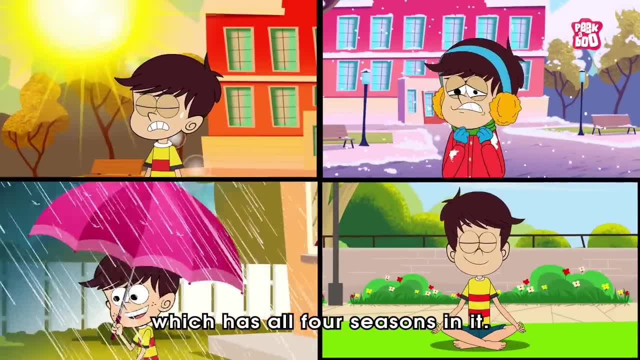 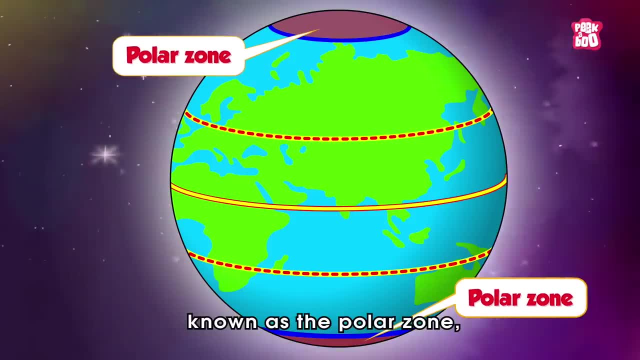 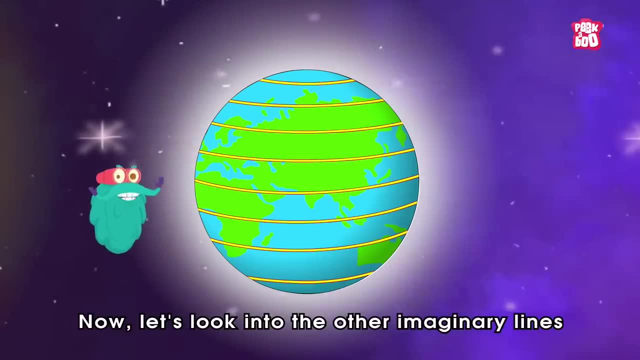 Which has all four seasons in it. And lastly, we have regions beyond polar circles, known as the polar zone, Where the climate is wintry and snowy due to lack of sunlight. Now let's look into other imaginary lines. we call longitude. 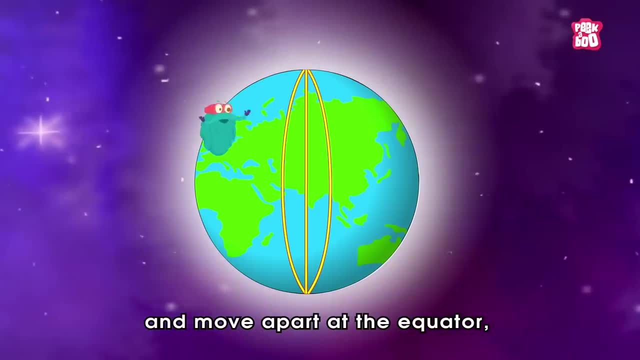 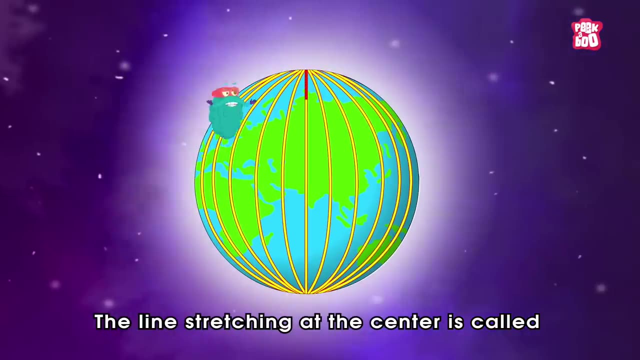 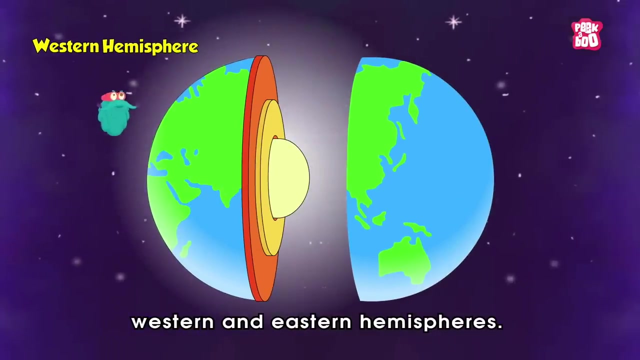 That starts from the top pole and move apart at the equator, Just to meet again on the other pole at the bottom. The line stretching at the center is called the prime meridian, Which divides the earth into western and eastern hemispheres. 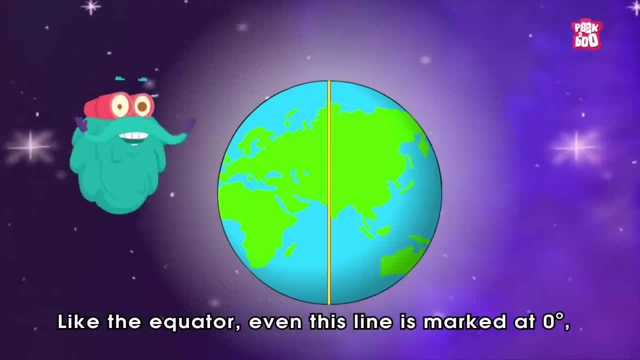 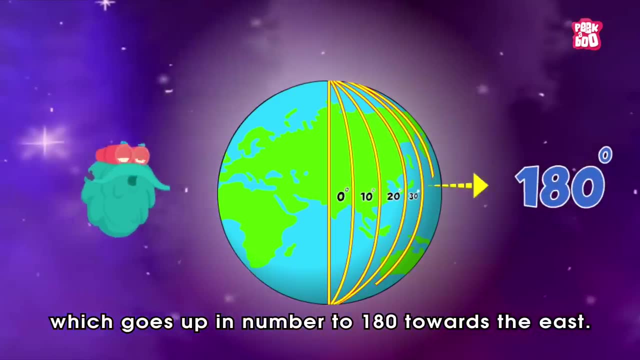 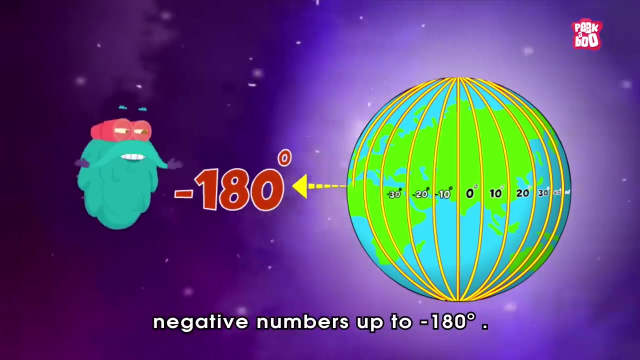 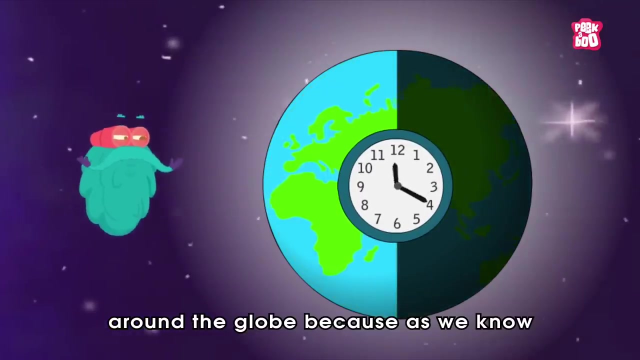 Like the equator, even this line is marked at 0 degrees, Which goes up in number to 180 towards the east, Whereas to the west it is denoted with negative numbers up to minus 180 degrees. These lines help in determining the time zone around the globe. 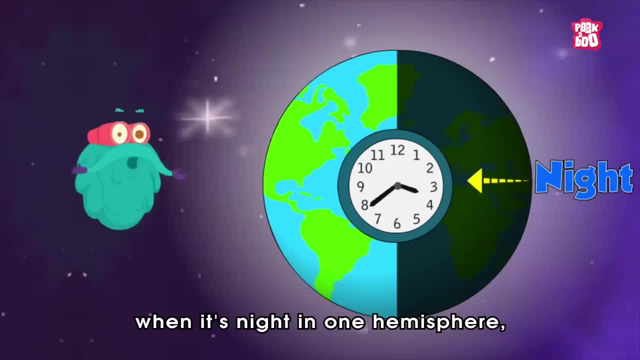 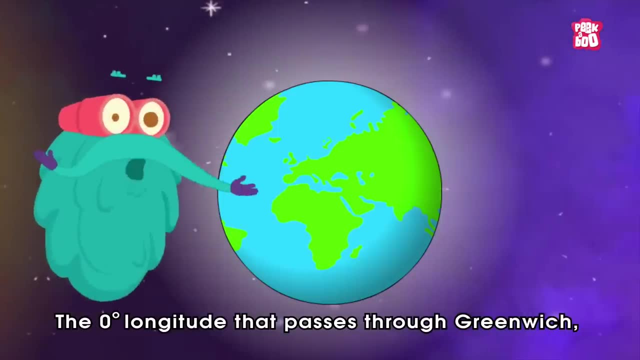 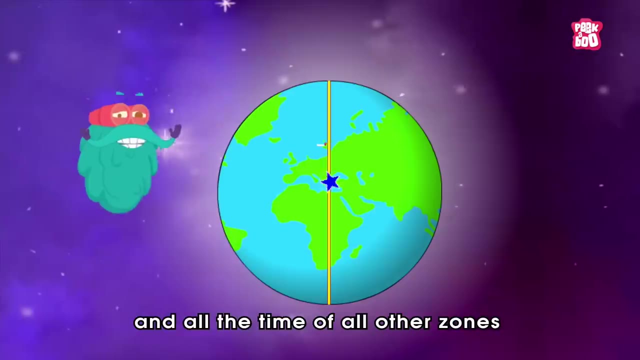 Because, as we know, when it's night in one hemisphere, it's daytime on the other part, and vice versa. The zero degree longitude that passes through Greenwich, near London, is considered a standard, And all the time of all other zones are calculated accordingly. 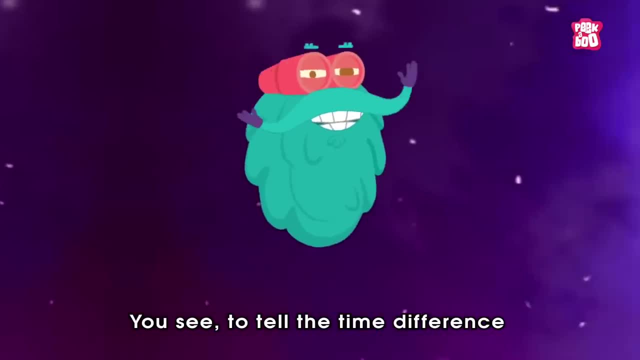 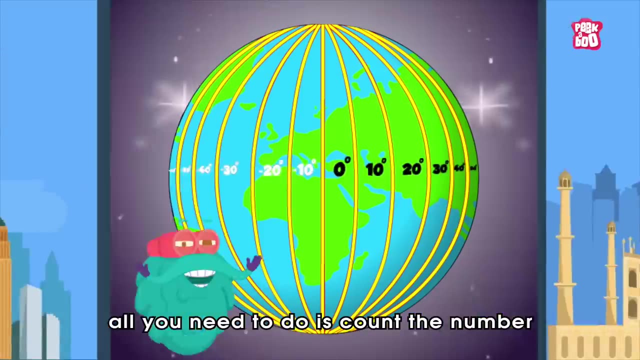 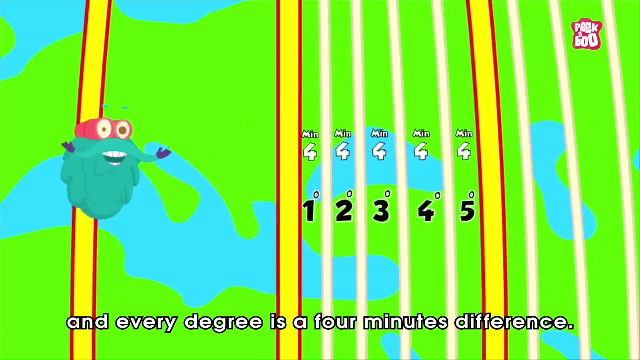 How? Let me explain. You see, to tell the time difference between two places, All you need to do is count the number of longitude degrees between them, And every degree is a 4 minutes difference. So if it is 12 noon at Greenwich, which is at 0 degrees, 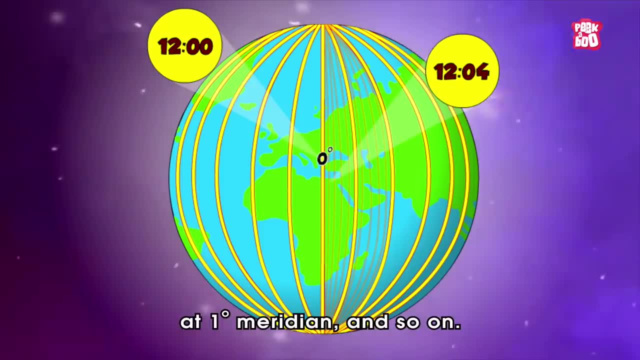 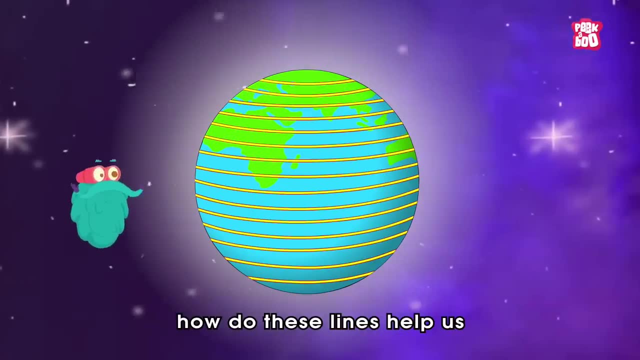 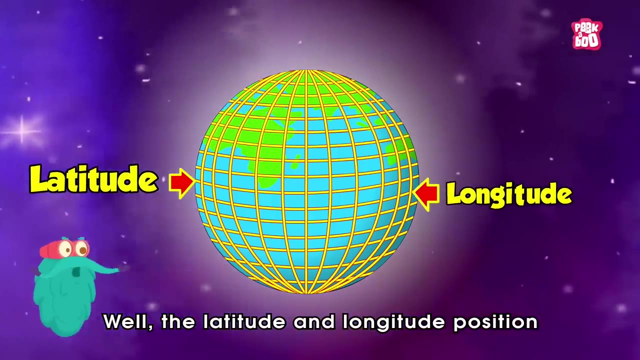 Then it will be 12.04 pm at 1 degree meridian, and so on. But the vital question is: how do these lines help us locate a place on the map? Well, the latitude and longitude position of any location in the world is known as its coordinates.